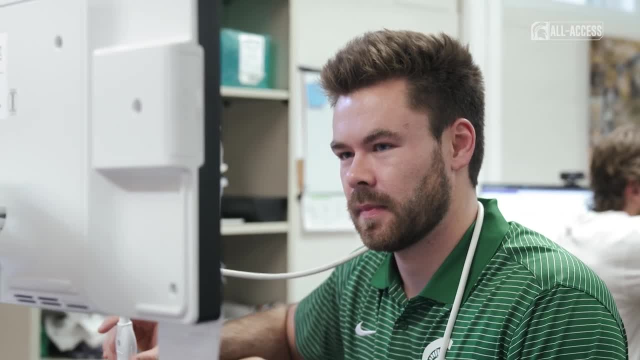 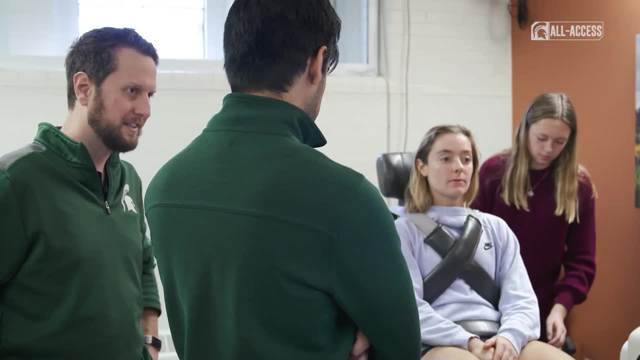 combining all of this together, all of our expertise, to really answer some of these questions about what we're doing and what we're trying to do. It's about long-term health, but also giving back to our student-athletes here and hopefully allowing them to be as best as they can be. 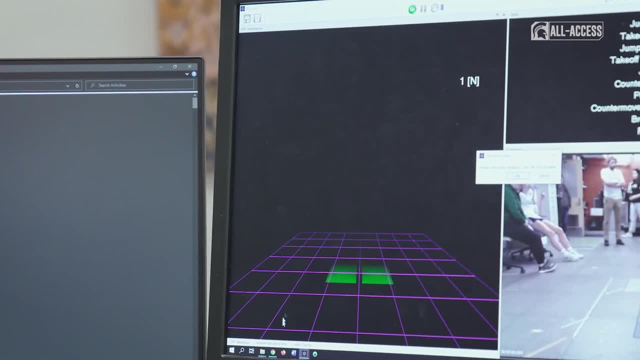 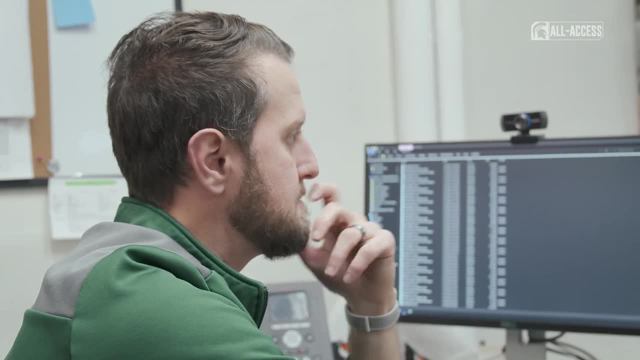 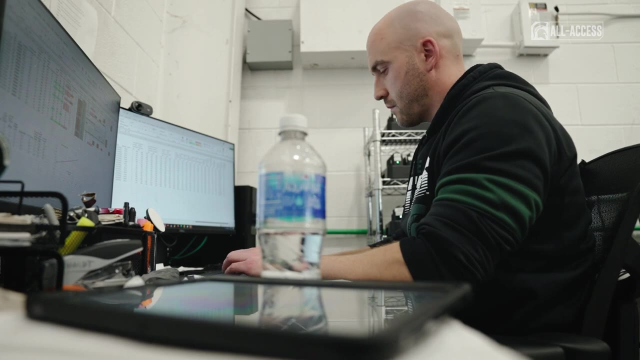 So what it allows us to do is have a resource, someone that is outside. they can see the latest trends in other sports. think about how that may apply and help us. Professor Harkey with kinesiology as a researcher and brings very much a biomechanist and a research focused emphasis to what we do and that helps us. 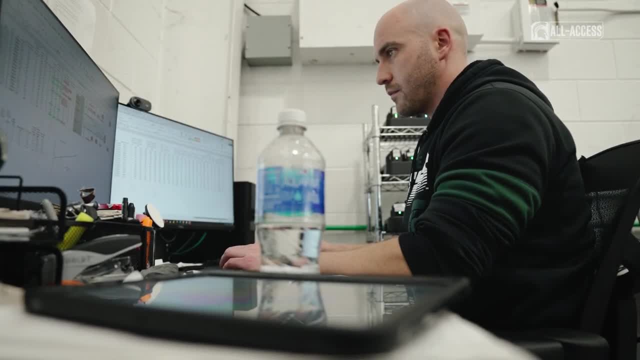 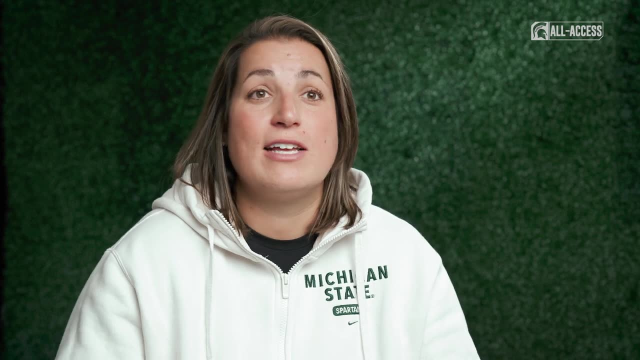 get the best information. We're looking at the best information that we can for our athletes, Where we're looking at muscle discrepancies or we're looking at and balances with players for quad to hamstring ratio, which is then driving our decision making in the weight room and the training room for kind of our Prehab as well. 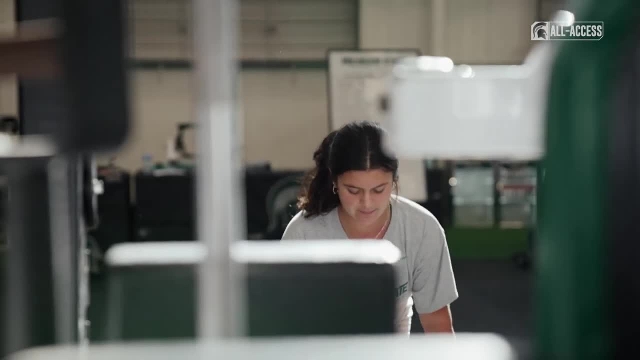 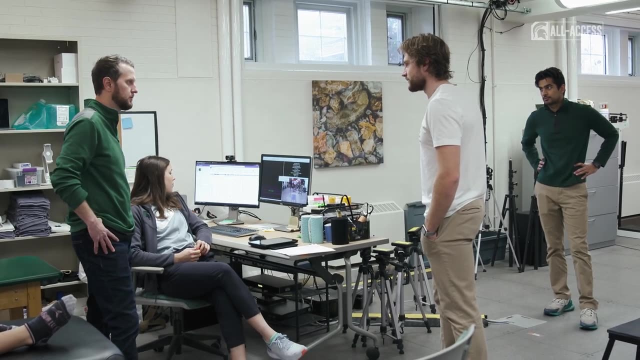 as our Rehab and really individualizing player development, a player growth which I think we're doing at a level that others aren't. We have put a big emphasis on collaboration, knowing we have experts in the field leaning on them. It doesn't matter if they're in the athletic department or not, like in the 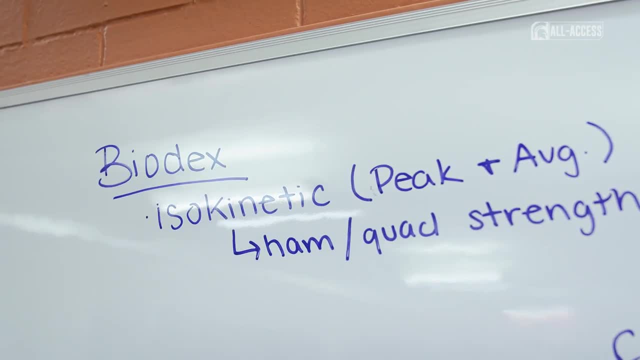 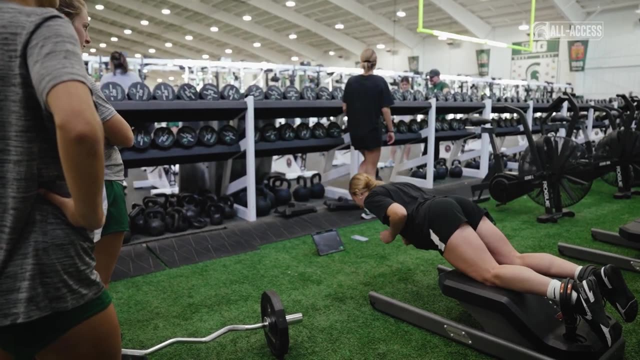 with the mission of giving our athletes the best environment as possible, then we exhaust all avenues to do that, and that's really where that's, top down, from your athletic director, down through your coaches and into your athletes. our athletes are more than willing to cooperate with what we're. 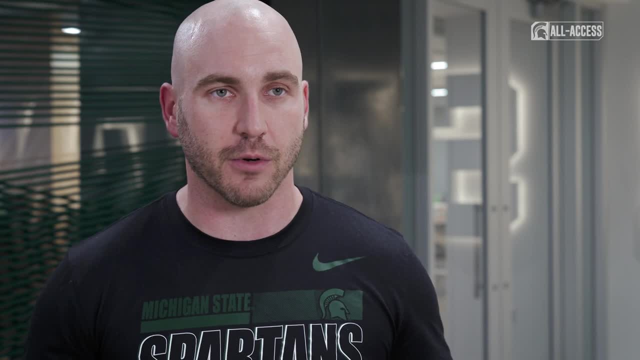 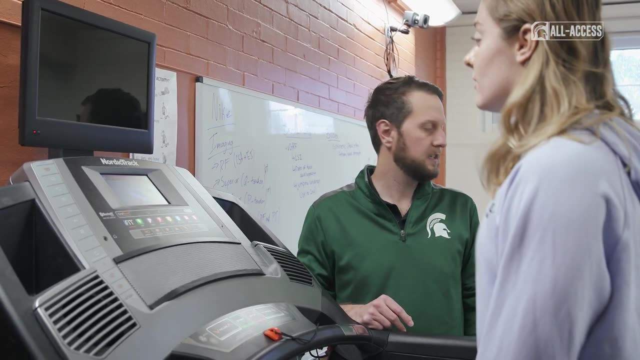 doing and are really asking a lot of questions and very engaged with what we're doing and where they're excited about the data that they're receiving on their end and just building that trust and helping push their training to the next level. i mean, it's been fantastic. 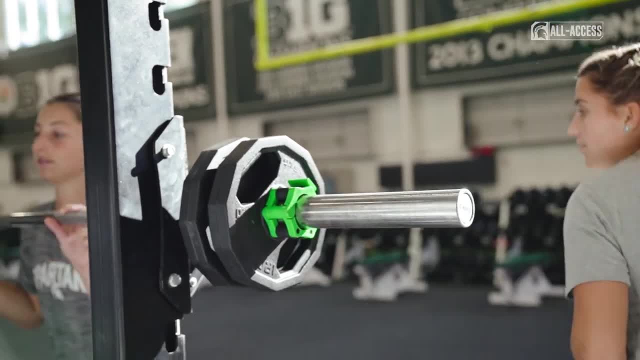 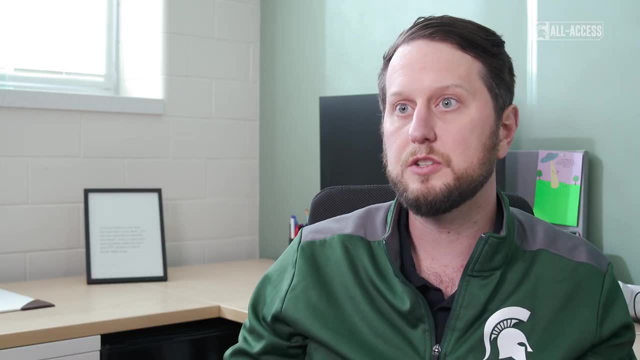 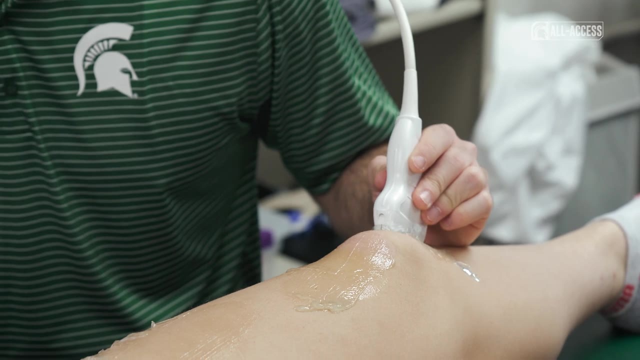 my specific research is trying to understand why people following knee injuries are at risk for arthritis. so some of these techniques are trying to look at kind of the long-term health of the joint, to see if is anything that these athletes doing kind of putting their joint and creating some type of structural 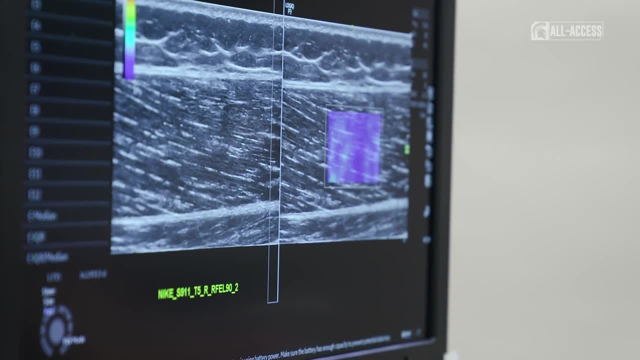 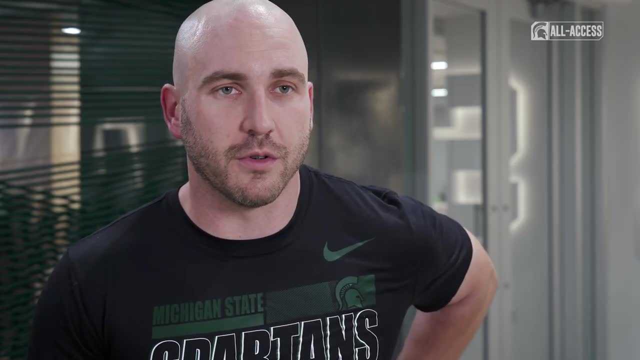 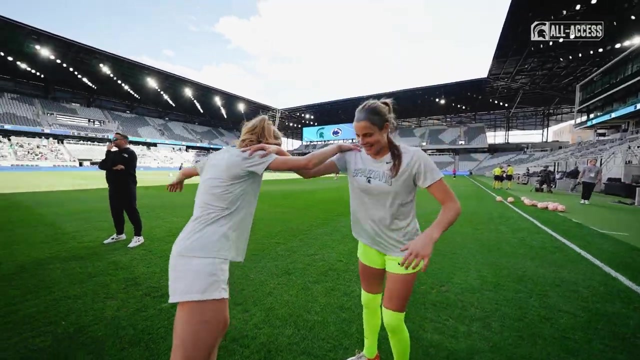 change that that may set them up for arthritis or some other long-term decline in health. most coaches will will tell you that the greatest ability is availability, right? so how can we uh get them to play at their best if they're not able to practice, if they're not able to train, if they're 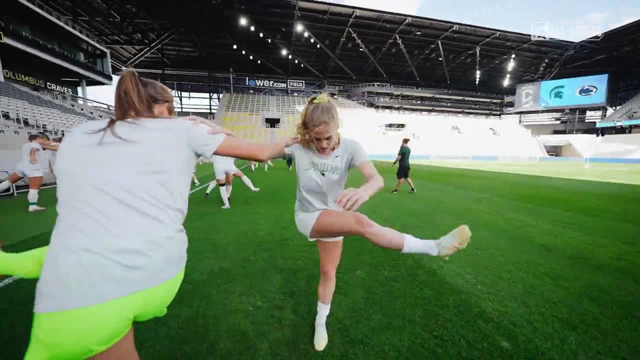 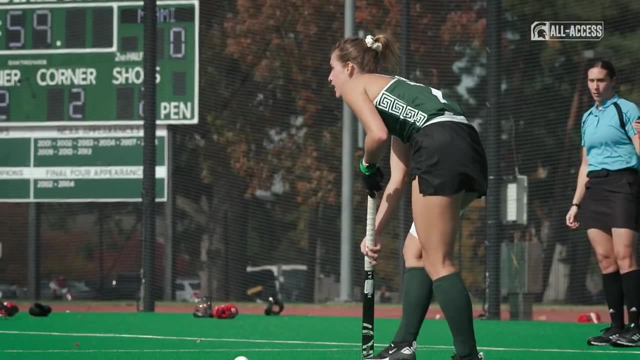 not able to actually be out on the field on on game day. so that's that's what we need them the most. so how can we reduce the risk of injury as much as we can, knowing it'll never be zero? but how can we just ensure that we're giving them the best chance to compete at the highest? 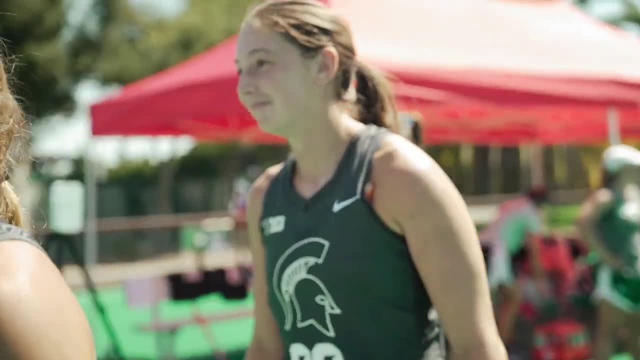 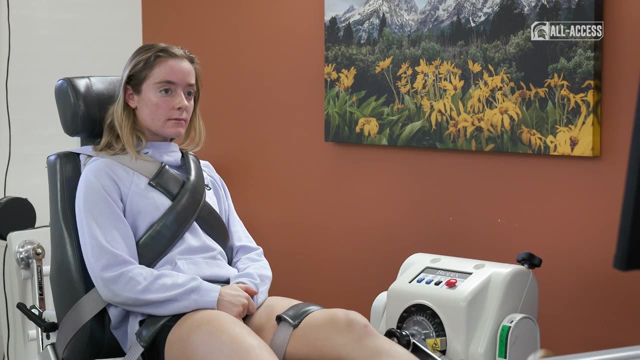 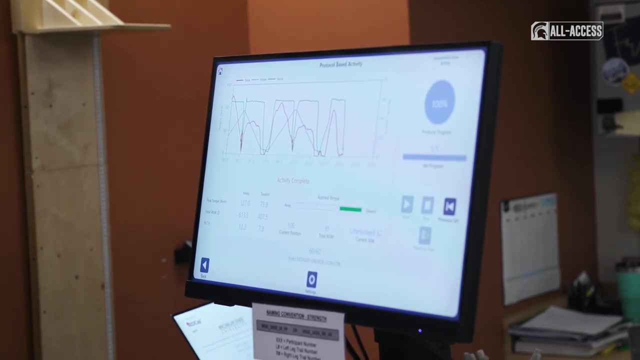 level for their sport. what can we do and what techniques are we doing to be able to identify athletes at risk for injury? that's kind of. the ultimate goal is to use some of these different tools where- whether it's the ultrasound imaging, the jump landing, biomechanics, the gps monitoring- what are these different pieces of the puzzle that we can? 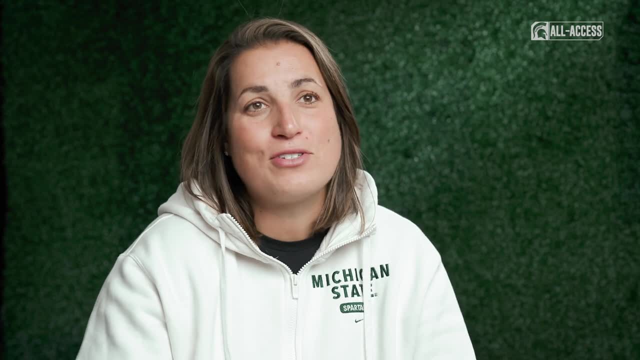 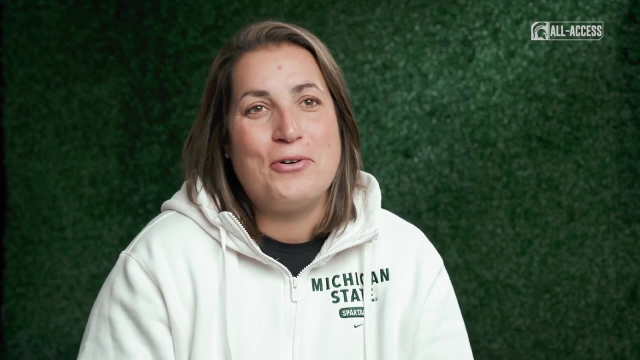 put together to understand who's at risk. Jim Pignataro was kind of the the person behind all this, and so for him not to be here to see this kind of playing out. you know, i know he'd be proud looking at where this has evolved and moved to, and i think that our sports science department as a 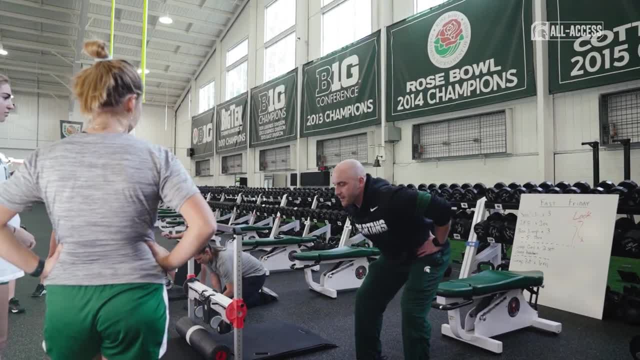 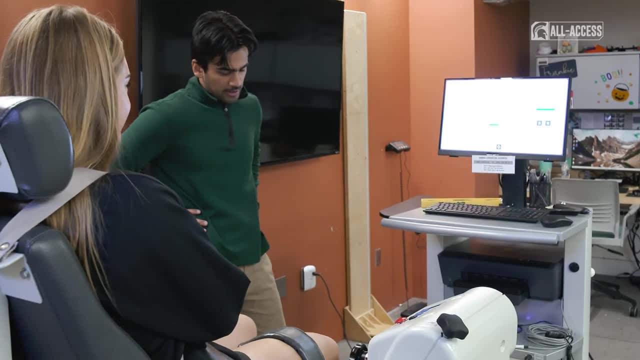 whole, with Bill Burkhart who's kind of leading the charge. we've got a lot of people that are full-time staff members, that are grads master students, that are here putting their time and energy into this and they're passionate about it. they love the numbers, the data, the information. so 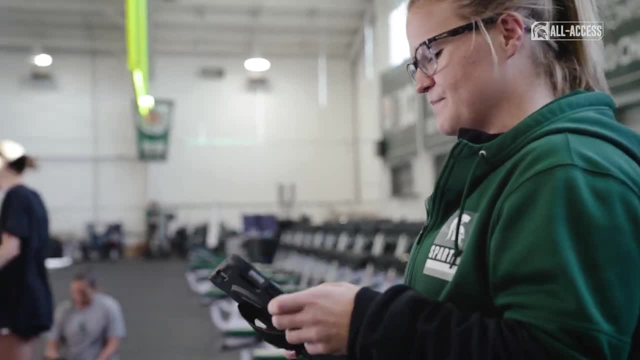 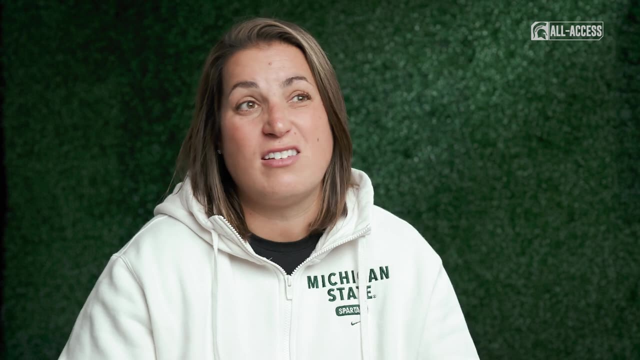 i think we are in the front edge of this and i think we're going to see more people that want to get on board to what we're doing, from institutional level to companies such as catapult or others that we're using for our wearables. i think we're only going to see it. 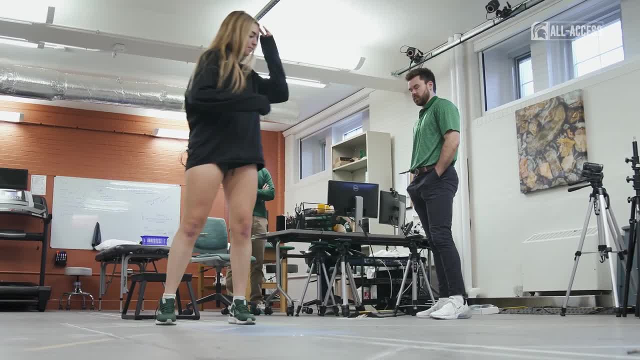 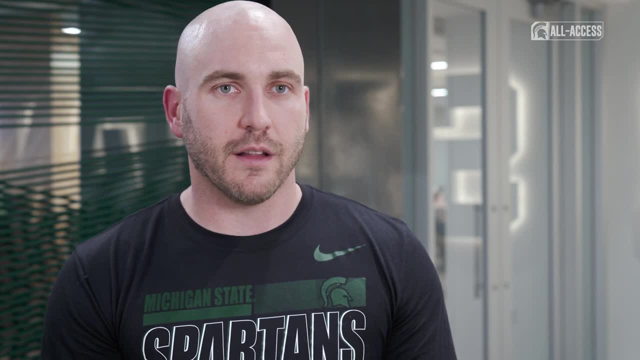 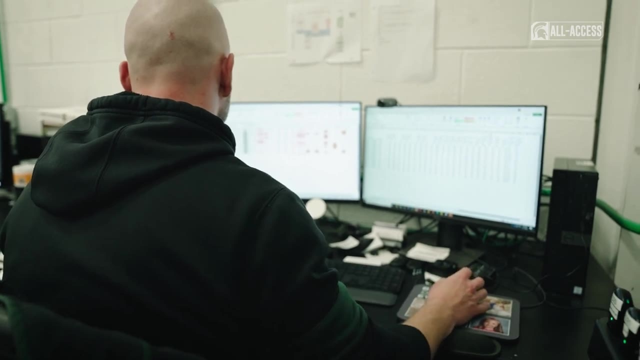 keep growing. our collaboration will probably always be ongoing. it's been mutually beneficial for everyone. my vision is that when an athlete steps on this campus, they can be assessed, we can know exactly what they're bringing when, wherever they're coming from, and we can design and implement the proper program for them to help them perform at the level they want to perform. 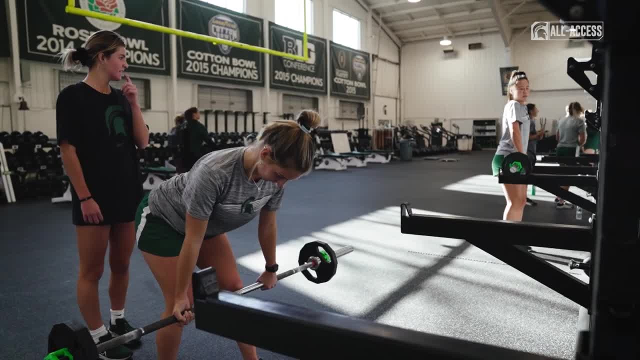 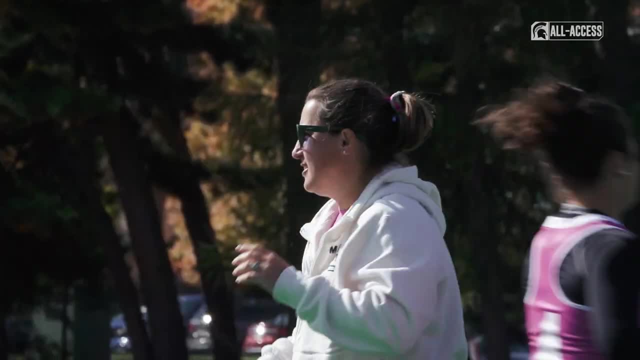 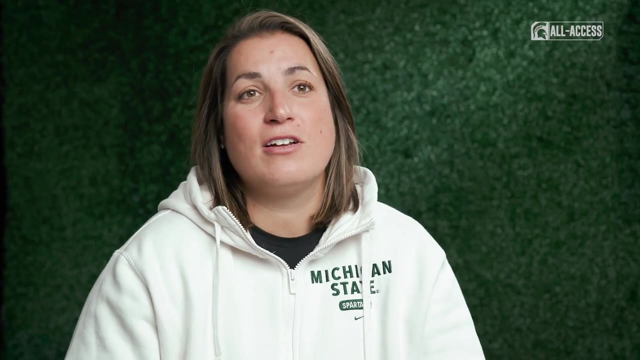 at and, should anything happen to them from an injury standpoint, knowing that they have best of care to get them back as safely and as effectively as possible. i think it's just this evolution of athletics as a whole and i think for female athletes to feel empowered with their bodies and knowing how they can be better, and to me this is just. this can be.